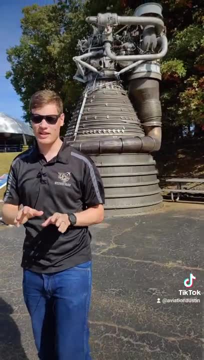 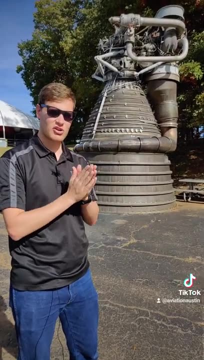 in order to move the nozzle of the engine. This movement controls the flight path in order to divert the exhaust in a way that can correctly position the rocket into its intended flight path. 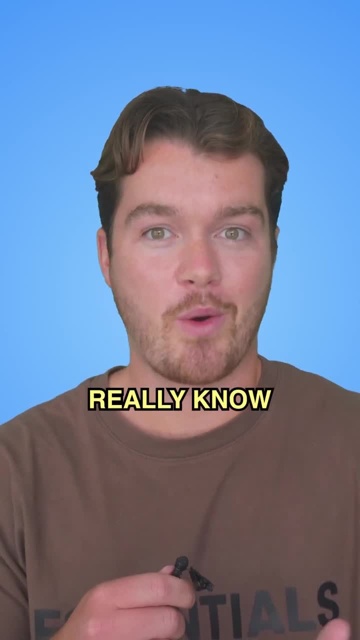 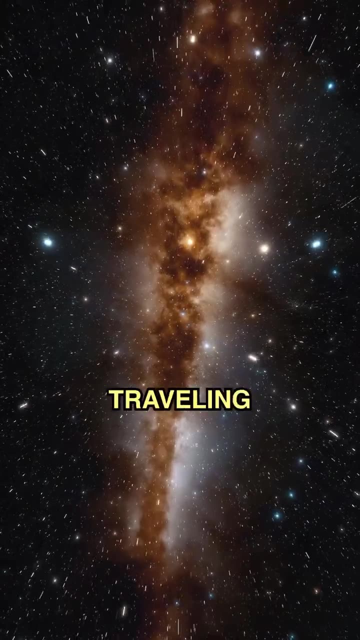 Where life came from is one of the biggest mysteries in the universe, because we don't really know how a bunch of molecules came together and then one day just came alive. But what if microbial life is not only abundant in the universe, but actually traveling through? 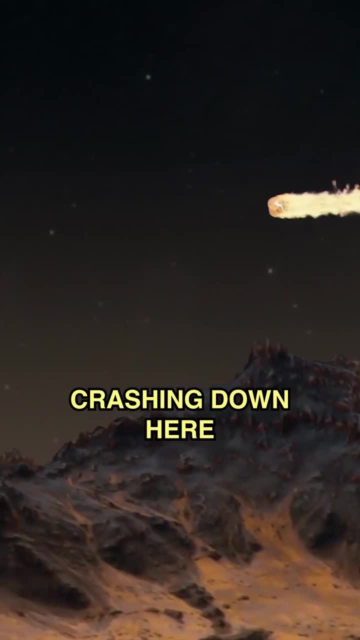 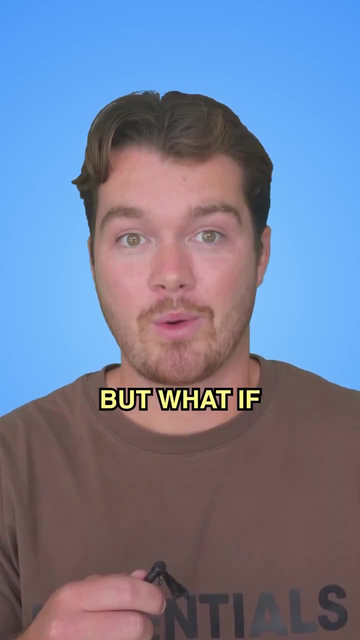 it. Here's what we know. Earth has water thanks to tons and tons of icy asteroids crashing down here billions of years ago, and our main theory is that somewhere in this water, probably in a hydrothermal vent, life just found a way. But what if life hitched a ride here on top of one of those? 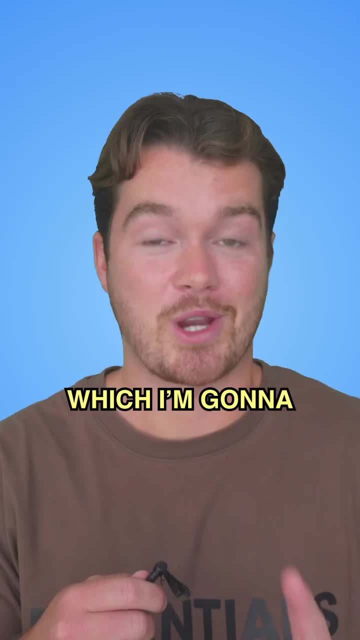 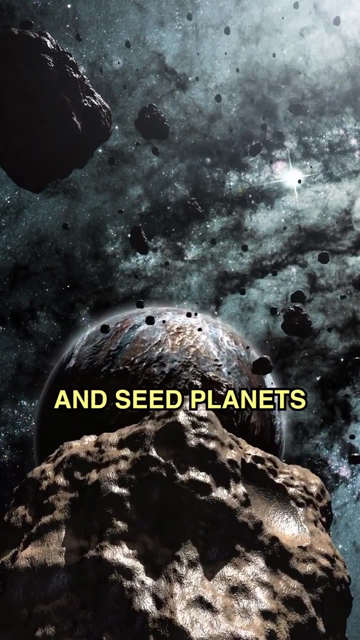 asteroids. I first heard about the Panspermia theory in the book Project Hail Mary, which I'm going to talk about in my upcoming book series, but essentially it's the idea that certain microscopic lifeforms can not only survive but travel through space and seed planets along the 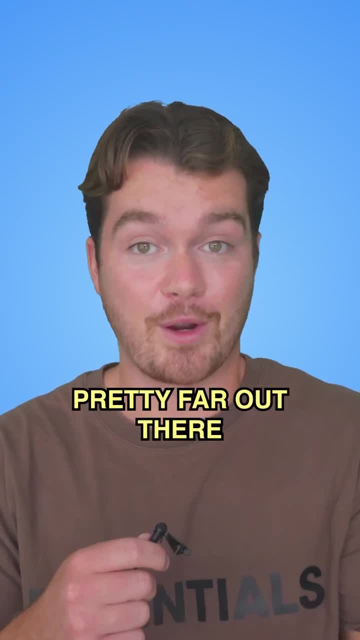 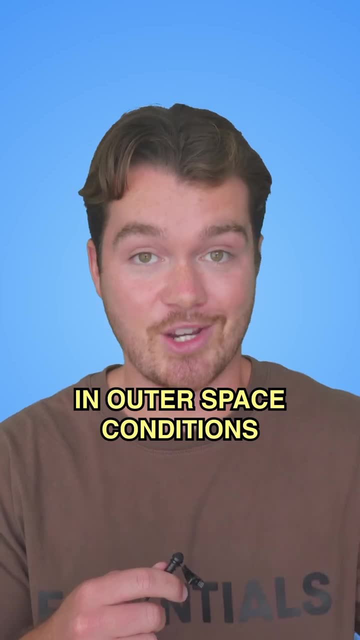 way, And that's where all life on Earth started. Now, this was a pretty far out there theory until scientists at the University of Tokyo found that a certain type of bacteria that I can't pronounce could potentially live up to eight years in outer space conditions. Eight years is long enough to 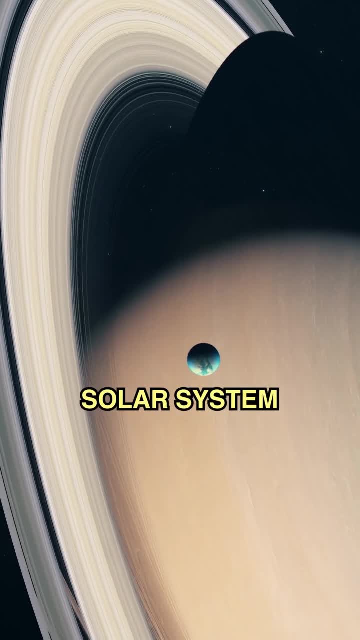 get to both Mars and Titan, two of the most probable locations for life in our solar system. so it's not impossible. Now again, this is just a theory, but if we could prove that either Mars or Titan have or once had a life form, then we could be sure that life on Earth would be.